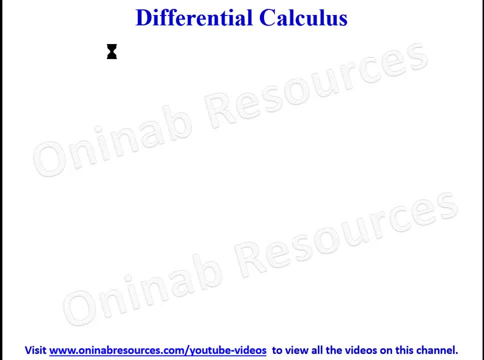 Hello out there. welcome to this tutorial again on differential calculus. In this video we'll be looking at product rule. Given the functions v equal to f of x, u equal to g of x and y equal to uv, then the y dx is equal to u dv dx plus v du dx. 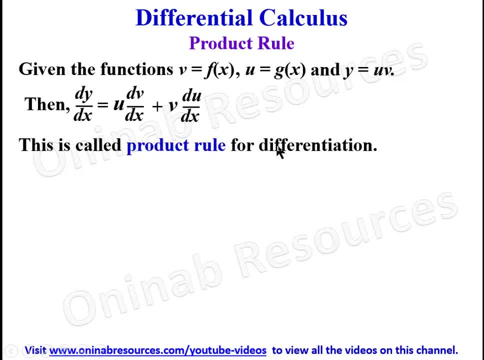 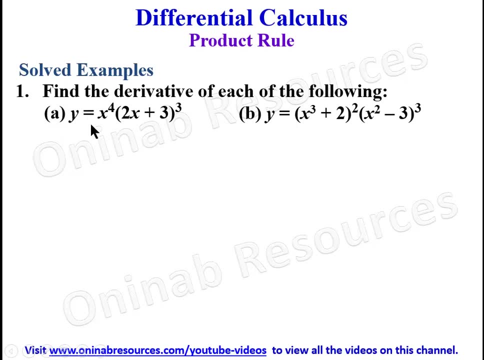 This is called product rule for differentiation. We take some examples on product rule for differentiation. So our first problem: find the derivative of each of the following: In problem a we have a product of two functions there. In problem b also, we have a product of two functions. So we are going to use a product rule. 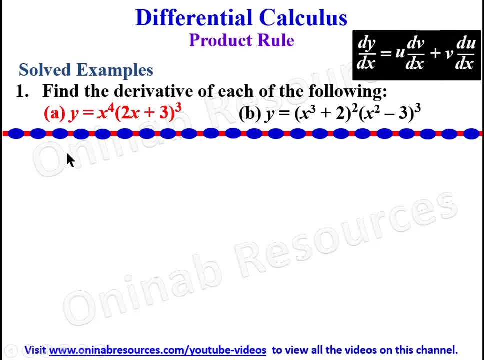 This is the product rule. here, Starting with problem a, we are going to identify function u and v so that we now have it as u equal to x raised to the power 4.. And from there we can find the u dx. The u dx here is: multiply the power by the function. 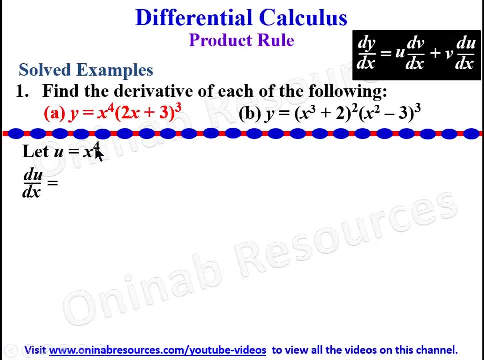 That will give you 4x. Then reduce the power by 1, which will give us 4x to the power of 3.. Then we let the second function to be equal to v, That is, we let v equal to 2x plus 3, all to the power of 3.. 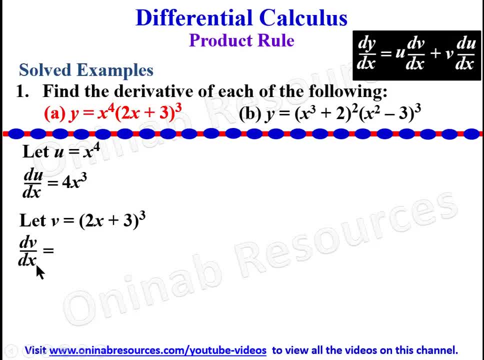 Then we differentiate. We find the v dx. We differentiate what we have inside the brackets: 2x plus 3.. The derivative of 2x is 2.. And the derivative of this 3, which is a constant, is 0. 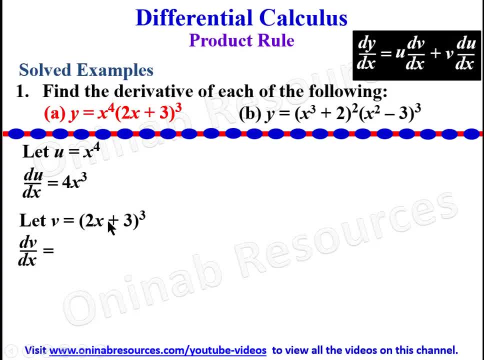 So we have the derivative of what we have inside the brackets to be 2.. Multiply it by the power, which is 3.. 2 times 3 will give us 6.. Then we pick the whole brackets, Then we reduce the power by 1.. 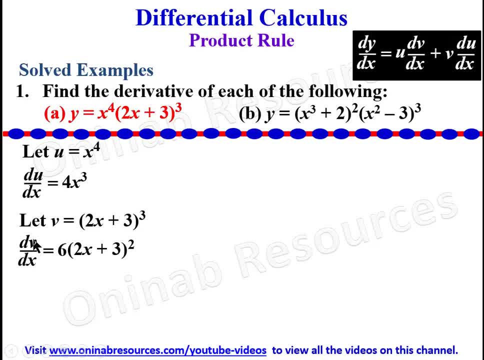 That's 3 minus 1, which will give us 2.. Therefore the v dx is 6 into 2x plus 3, all to the power of 2.. So from here we can find the y dx based on this product rule. 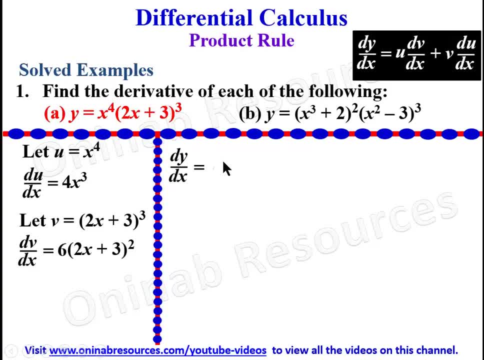 So we have u. Where is our u? This is x raised to the power 4.. The v dx: The v? dx is 6 into 2x plus 3, all to the power of 2.. Therefore we have it times 6 into 2x plus 3 to the power of 2.. 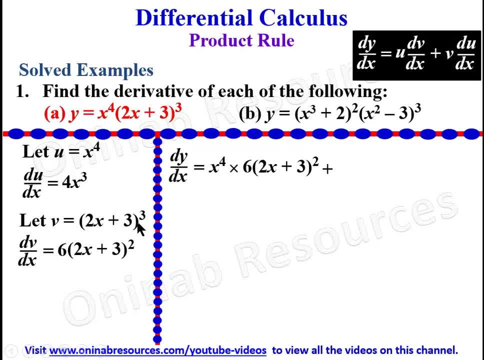 Then, plus what is our v? This is our v, So we have our v here. Then we bring in the u dx. The u dx is 4x cubed, So we have it as times 4x cubed. So, having gotten this, 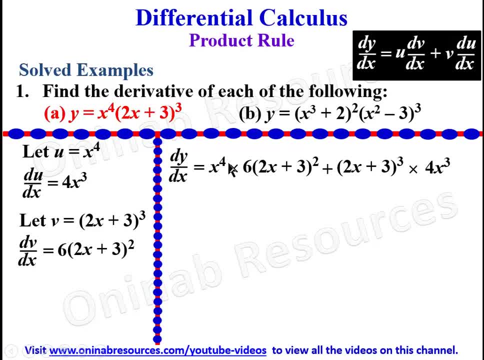 we simplify: x raised to the power of 4 times 6.. We give us 6x raised to the power of 4 into 2x plus 3, squared plus 4x, cubed into 2x plus 3 to the power of 3.. 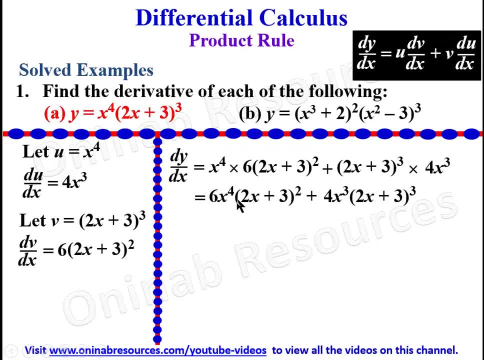 Then we can factor out this: This is 6x to the power of 4.. 4x to the power of 3.. We can get 2x cubed here, 2x cubed here. So between this and this, 2x cubed is a factor. 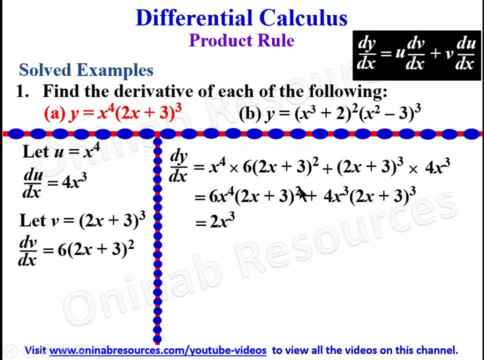 Then, between this and this: this is to the power of 2, this is to the power of 3.. So 2 to the power of 2 is a factor. So we have 2x plus 3 all squared. Then we now go ahead. now to 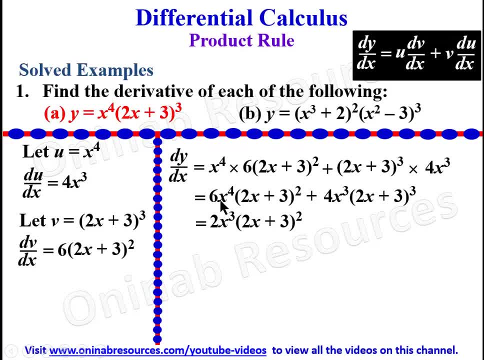 factorize For this first part: 6x to the power of 4 divided by 2x. cubed 6 divided by 2 is 3.. x raised to the power of 4 divided by x raised to the power of 3, will give us x. 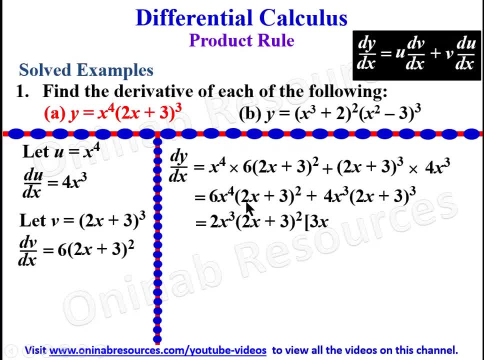 So we have it as 3x, And here this is to the power of 2,, this is to the power of 2.. So it gives 1.. So that's plus. So we go: 2x cubed, 4x cubed. 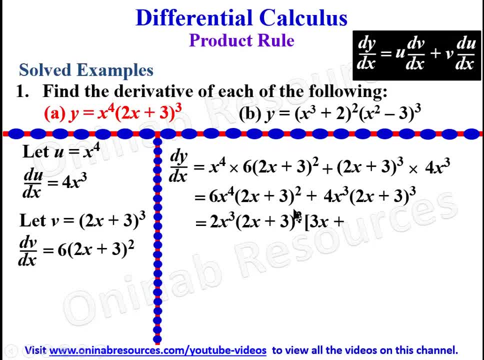 4x cubed divided by 2x cubed, We have 2 there, And this is 2x plus 3, all to the power of 3.. Dividing it by 2x plus 3, all to the power of 2.. 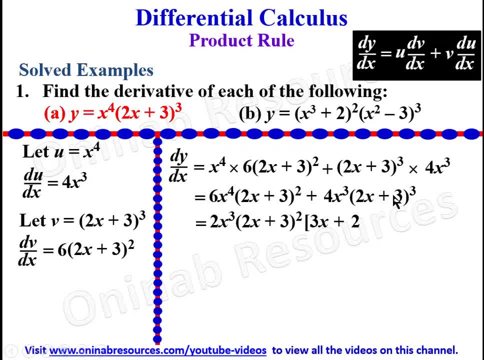 So this 2 will cancel. This 2 will be left with 2x plus 3.. And we still maintain the first two factors. So we maintain the first two factors. We simplify this: This is 3x here. 2 times 2x will give us 4x. 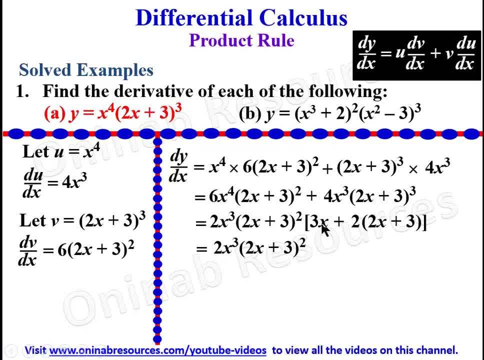 So 4x plus 3x will give us 7x, So we have 7x. And this is 2 times 3 will give us 6.. So we have it as a plus 6.. This is the derivative of the function in problem 1a using the product rule. 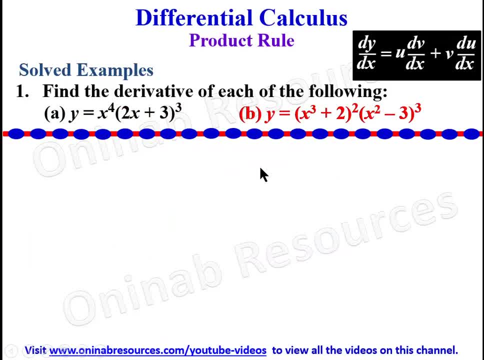 So we go to problem 1b. For problem 1b, again, we have to identify u and v. So the first part. For your information, your choice of u or v does not affect the result of this derivative. So if you like, you can take this one as v. 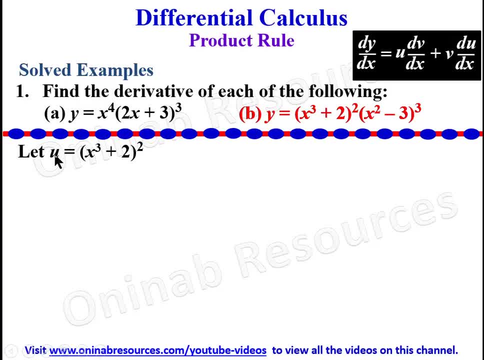 You can take this one as u, It doesn't matter. We let u equal to x, cubed plus 2, all to the power of 2.. Then we find the u dx. So the u dx will be differentiating what we have inside this bracket. 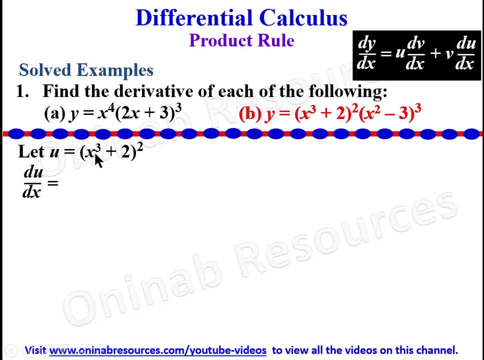 Multiply by the power, Bring the bracket, Reduce the power by 1.. So we go Differentiating. this will give us 3x squared, And the derivative of this constant is 0.. So the derivative of what we have inside this bracket is 3x squared. 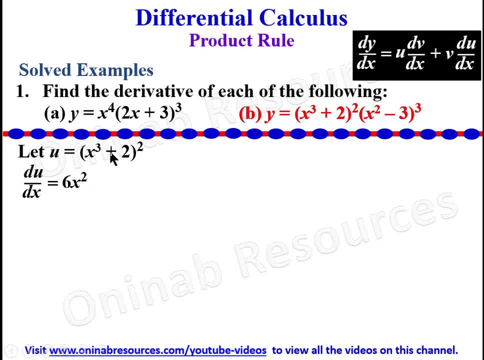 Multiplying by this power will give us a 6x squared. Bring the bracket, Reduce the power by 1. So we'll be left with 1.. So it doesn't make any difference. This is the derivative of u with respect to x. 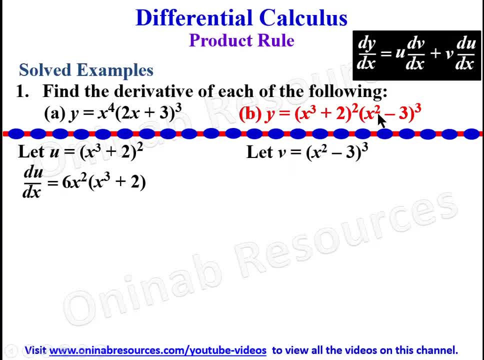 So also we let v equal to the second function. y is a product of two functions here, So we've taken the first one to be u, We take the second one to be v. Differentiating v with respect to x: The derivative of what we have inside the bracket is 2x. 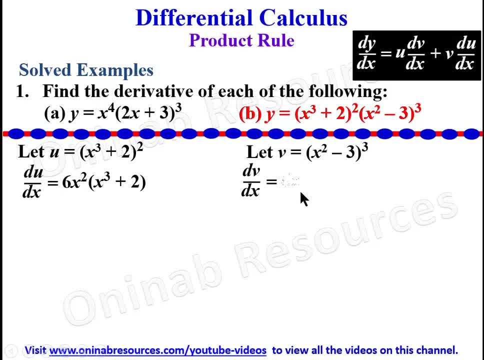 So, multiplying that 2x by this power, we have a 6x. Bring the bracket, Reduce this power by 1.. We have a 2.. Therefore, the v dx is 6x into x squared minus 3r squared. So we now go ahead to find the y dx. 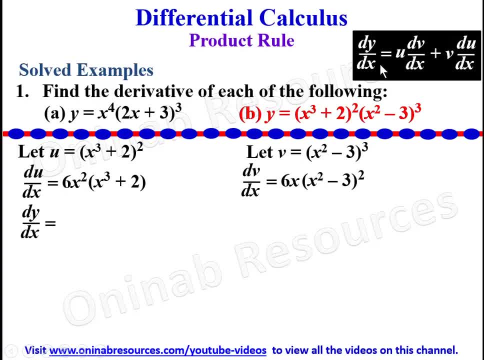 To find the y dx. We bring in u. Our u is this. So we have a u dv dx. This is dv dx. We bring in dv dx. We have dv dx 6x into x squared minus 3r squared. 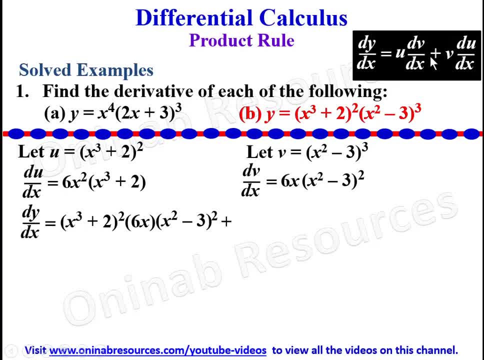 And the next thing is plus. Where is our v? Our v is this: We bring in v, Then bring in the u dx And our dv dx is this: So that is 6x squared into x cubed plus 2.. 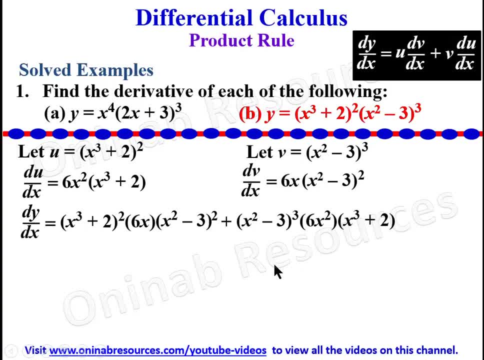 That's all. We now simplify this expression. Simplifying this expression, We look at this: 6x, 6x squared, What is the factor? The factor is 6x, So we keep the 6x. We check the first bracket here. 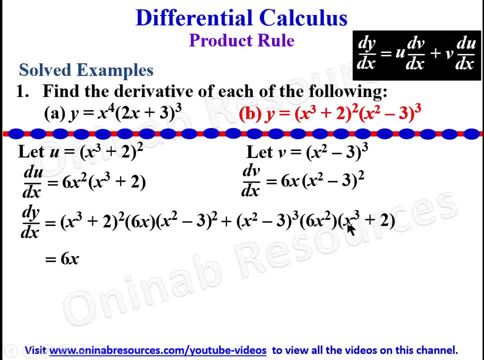 This is x cubed plus 2 to the power of 2.. x cubed plus 2 to the power of 1.. So the factor between this and this is this one with a power 1. Which is x squared plus 2.. 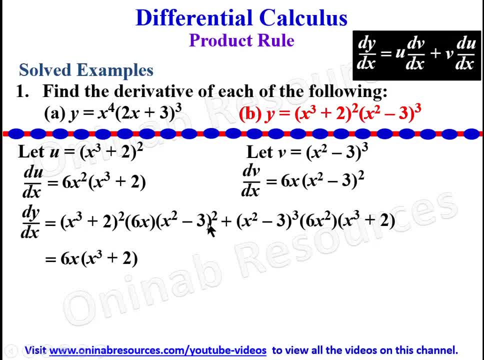 Then we come here. This is x squared minus 3, all to the power of 2.. This is x squared minus 3, all to the power of 3.. So this is a factor between this and this. So x squared minus 3 to the power of 2.. 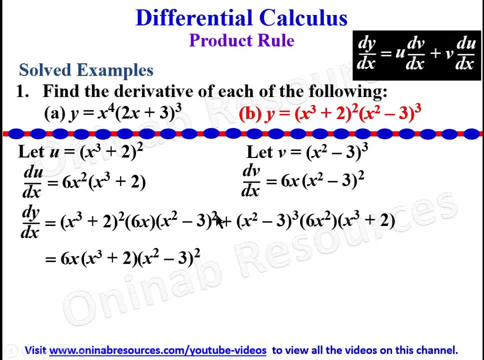 Now we go ahead to divide this, The first part of this expression, by this, Taking it one after the other: 6x divided by 6x is gone. Now give us 1.. This is x cubed plus 2, all squared divided by x cubed plus 2.. 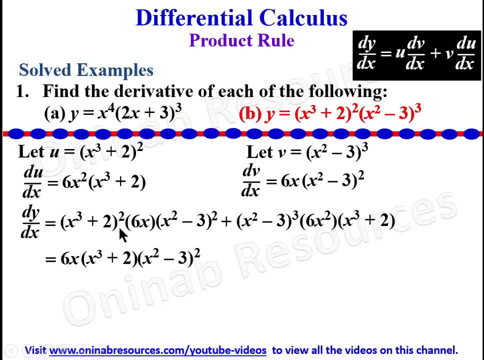 We will be left with x cubed plus 2. Only 1. That will give us x cubed plus 2.. Since this divides, this will give us 1.. Then, plus the whole of this now divided by this, 6x divided by 6x squared will give us x. 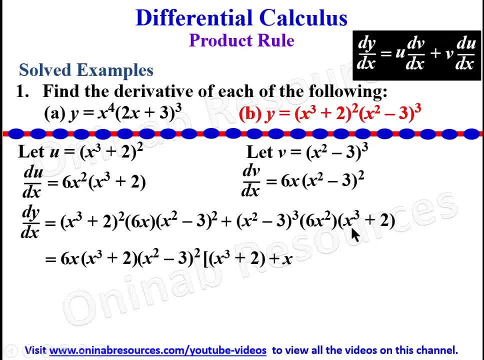 And x cubed plus 2. divided by x cubed plus 2 will give 1.. Now x squared minus 3, all squared, divided by x squared minus 3 cubed, We will be left with 1 of this as x squared minus 3.. 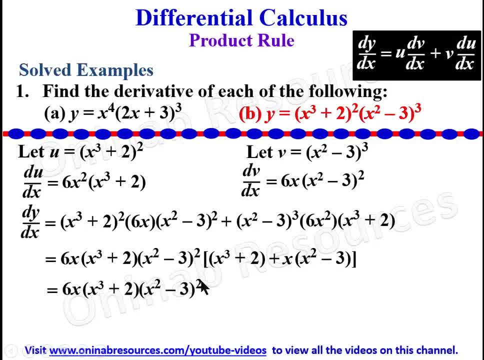 Then we now keep the first set of factors, And here this is x cubed plus 2. If you expand this bracket it will give you x cubed minus 3x. So the two like terms there are the x cubed and this x cubed when expanded. 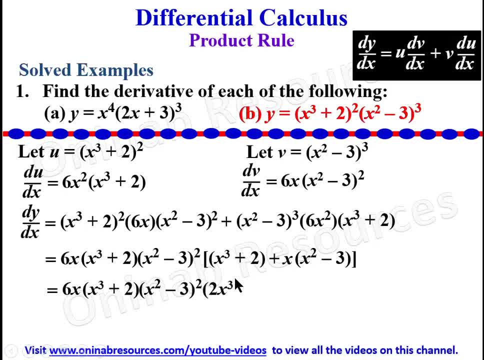 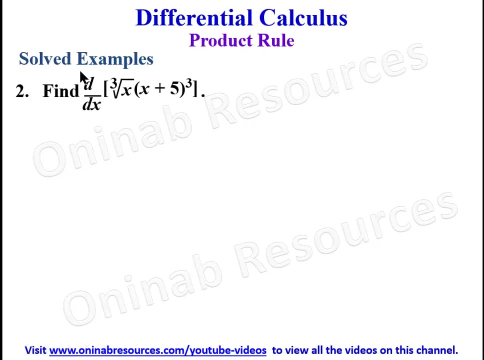 Adding them will give us 2x cubed. Then we have minus 3x here, Then plus 2.. This is the derivative of the second function in problem 1b. So we go to problem 2.. In problem 2 find the y dx of cube, root of x into x plus 5 to the power of 3.. 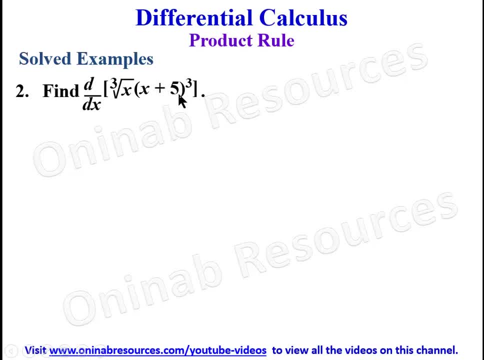 Again, this is a product of two functions. This is the first function multiplying this second function, And we are still going to use the product rule. Using the product rule, we are going directly here, But before we go, we need to write this cube: root of x in index form. 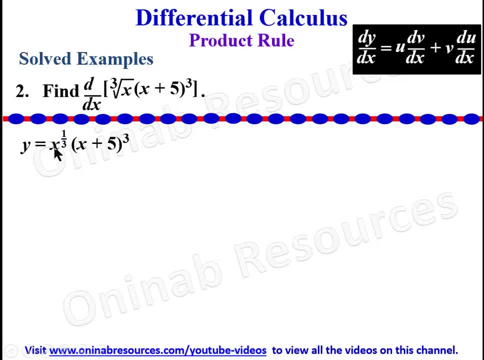 So we write this function as y equal to x, raised to power 1 over 3, into x plus 5 to the power of 3.. Now we are going directly here this time around, So we name this one u and name this one v. 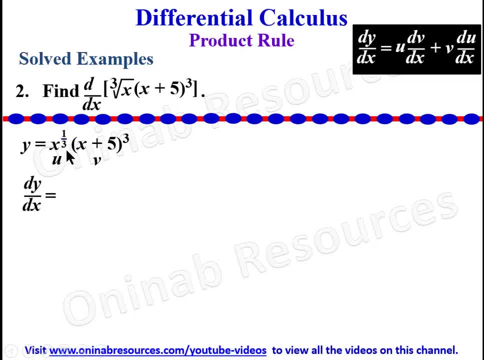 We have the y dx will be equal to u. We are keeping u, That's x raised to power 1 over 3.. Then the v dx. we differentiate this. Differentiating this, the derivative of what we have inside the bracket is 1.. 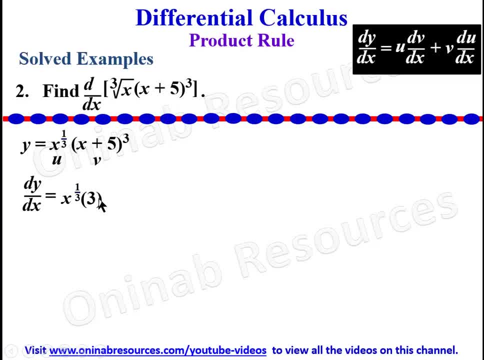 So multiply by the power will give us 3.. And bring the bracket, Reduce this power by 1.. That will give us 2.. We have gotten the first part of this derivative. Then to get the second part, that is going to be plus. 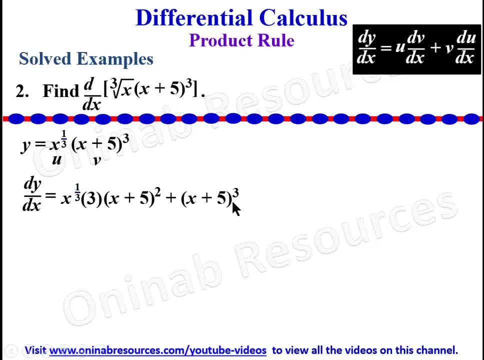 We keep v- v is x plus 3- to the power of 3.. Then we differentiate u with respect to x. So differentiating u will multiply by the power. that is going to give us 1 over 3.. 1 over 3.. 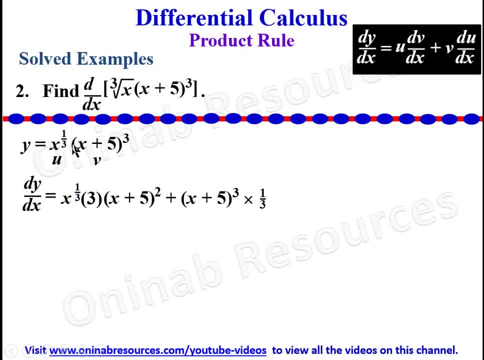 Reduce the power by 1.. 1 over 3 minus 1 will give us negative 2 over 3.. So that will give us x to the power of negative 2 over 3.. We can go ahead to simplify. I can revert back this to cube root of x for better simplification. 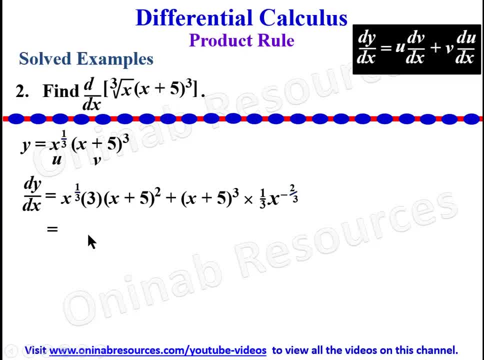 Multiplying it by this will give us 3 cube root of x Into x plus 5. squared Then plus x plus 5 to the power of 3.. I want to write this as fraction Because this is a negative index here. 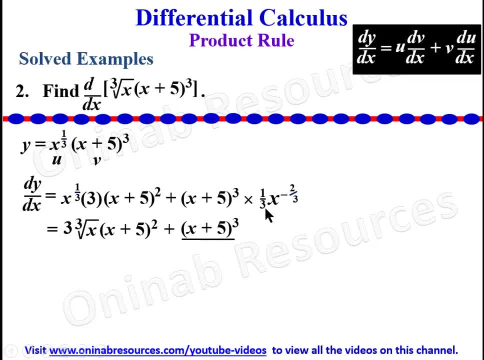 I will have it as 1 over 3 here, This 3. And this is going to form cube root: 1 over 3.. This one will form cube root, While this one will form square. So the whole of this now is 1 over cube root of x squared. 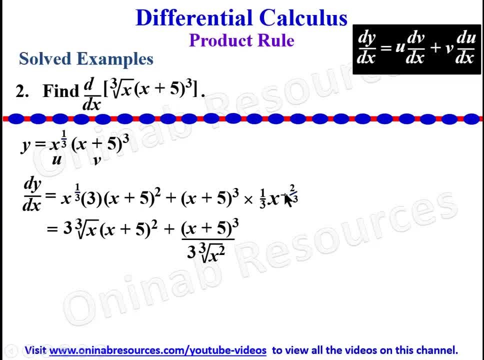 So we have it as cube root of x squared as the denominator, because of this negative index. So from here we make it a single fraction. The LCM is 3 cube root of x squared. So 3 cube root of x squared is the LCM. 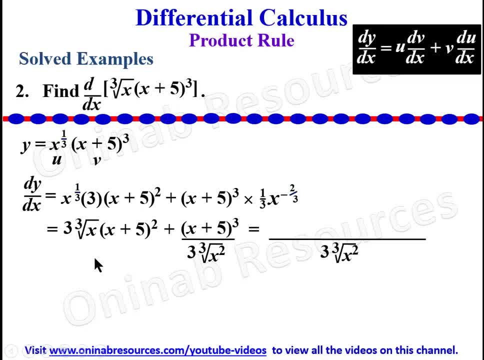 Remember this is over 1.. So this divided by the 1 there will give us 3 cube root of x squared. Multiply by this We do the multiplication bit by bit- 3 times 3 will give us 9.. Then this cube root of x is the same thing as x raised to the power 3.. 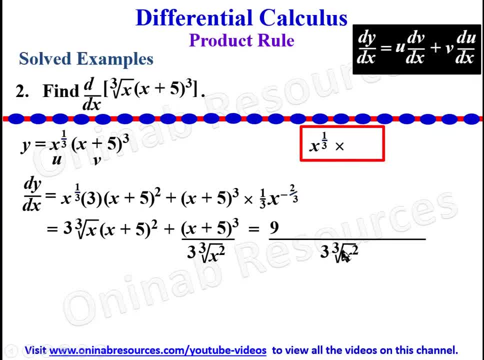 Times. this one is the same thing as x raised to the power 2 over 3.. Times x raised to the power 2 over 3.. 1 over 3 plus 2 over 3 will give us 1.. So from here we have x raised to the power 1.. 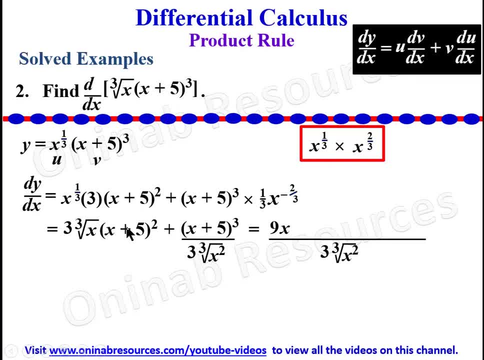 Which will give us x. Then we bring in this, That's into x plus 5 squared And plus, Since this divide, this gives 1. So we have the numerator maintained. Now We can simplify further By factorizing the numerator. 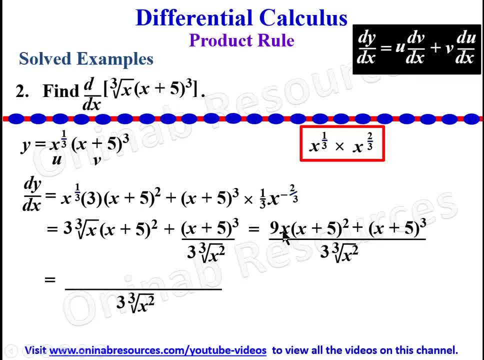 The denominator will still be maintained If we maintain the denominator 9x is not common. This is x plus 5 squared, x plus 5 cube. So this x plus 5 squared is a factor And Dividing this by this.